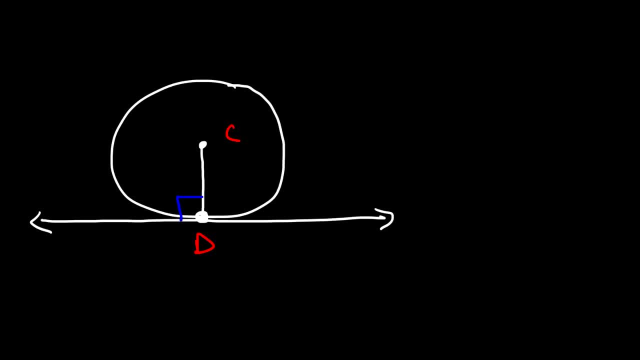 You need to make sure that you have a tangent line, need to know that these two are perpendicular to each other. they meet at right angles. Now there's another theorem with tangent lines that you need to be familiar with. So let's say, if we draw a tangent segment and another one, let's say that these two 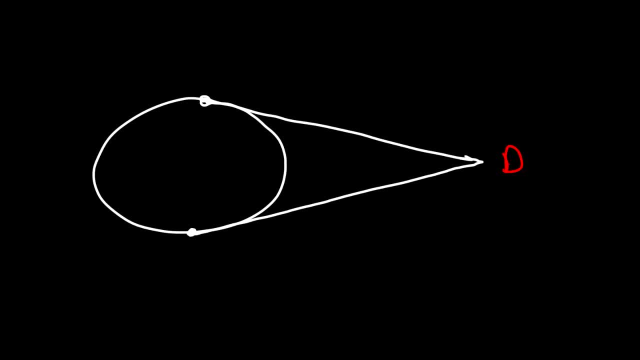 segments meet at point D, And this is point A, point B and we have center C. So if we draw two tangent segments from a common endpoint, point D, to the center of the circle, point C, then according to the two tangent theorem, the two tangent segments are congruent. 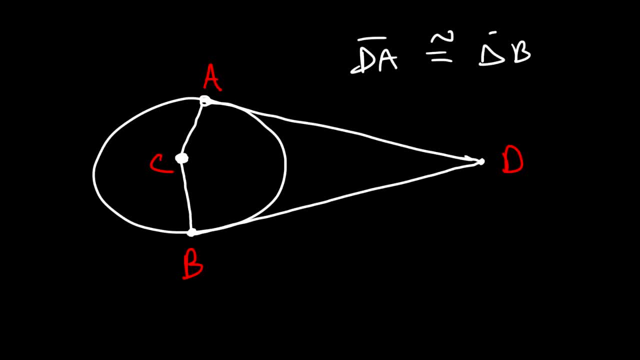 So DA is congruent to DU, C is congruent to CB. So this side is congruent to that side And you can prove it based on the hypotenuse leg theorem. So notice that we have two right triangles, because any time you draw the radius to a, 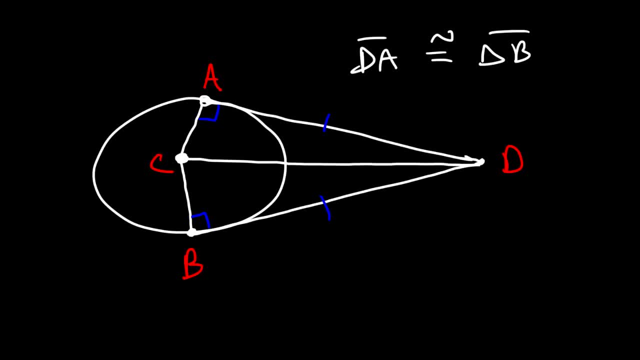 tangent line or even a tangent segment, it forms right angles And we know that AC has to be congruent to CB because they represent the radius of the circle, And then we have a common side, CD. So using the DHL theorem and also CPCTC, you can prove that DA and DB are congruent. 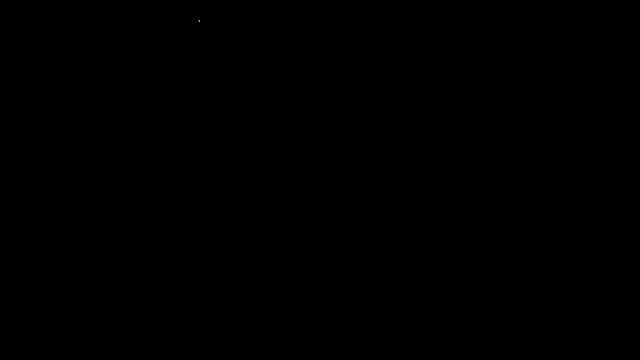 So that's the two tangent theorem. Now let's continue our discussion with something called tangent circles. Now you might be wondering: what exactly are tangent circles? So I'm going to draw two pictures for you. So I'm going to draw two pictures for you. 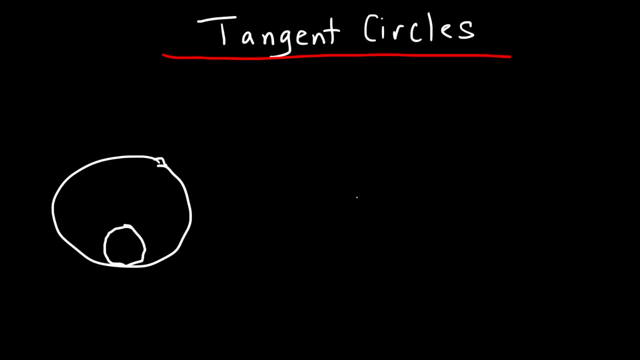 And then you think about what they mean. So that's an example of a tangent circle, And here is another example. So tangent circles- let's draw this line better. Tangent circles intersect each other at exactly one point, So notice that they both meet at the same or on the same tangent line. 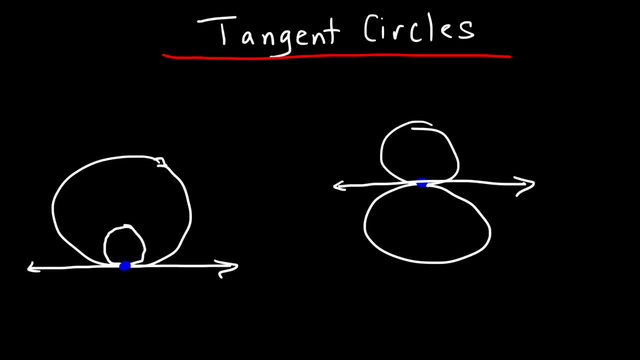 So these are tangent circles, And then you think about what they mean. So these are both tangent circles. Now what's the difference between these two circles? On the left, the two circles are internally tangent. So what does that mean? Two circles are internally tangent if one circle lies inside of another and if they. 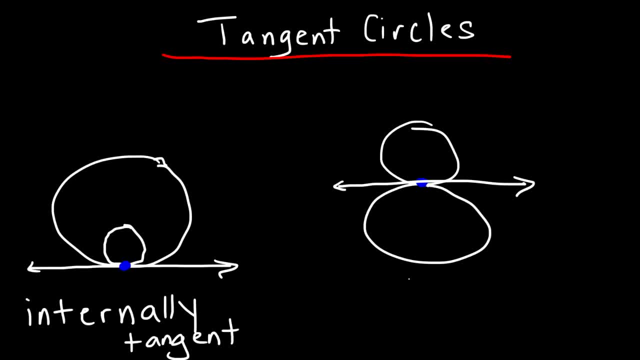 intersect at exactly one point, which they do. On the right side we have two circles that are externally tangent to one another. both lie outside of each other and they still intersect at exactly one point, but here they both one lies inside of the other, so just remember the word internal. 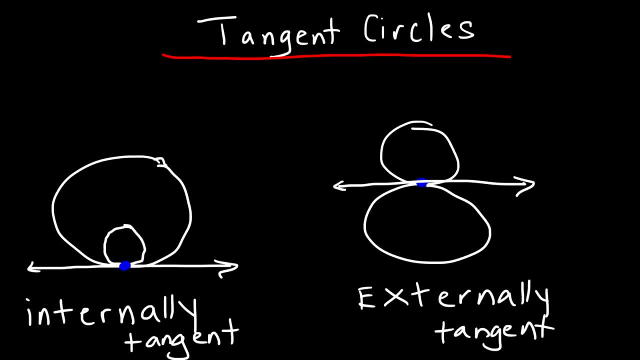 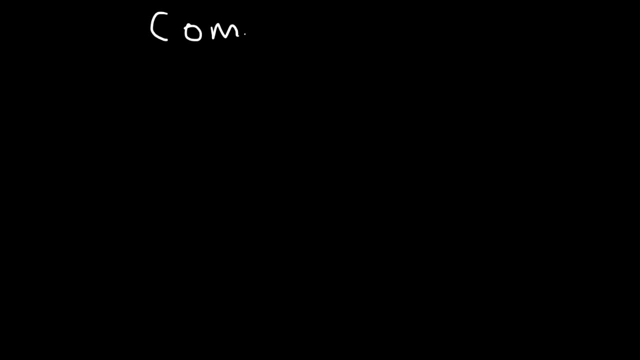 means to be inside of something. external is outside of something. so here one circle lies inside of another. it's internally tangent. here both circles lies outside of each other, so they're externally tangent. so let's talk about common tangents. what exactly are common tangents? a common tangent is a line that 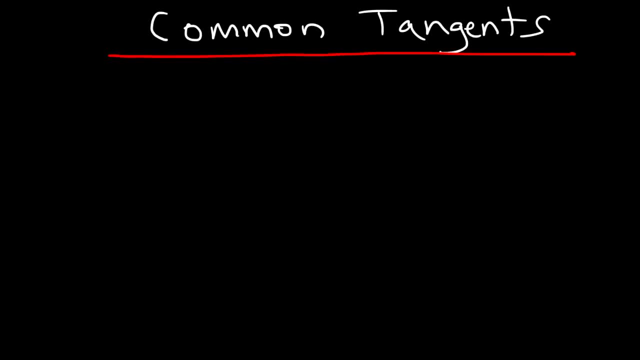 is tangent to two circles. now, it doesn't have to intersect the two circles at exactly the same point. the two circles simply have to be on the same tangent line, and so let me illustrate that. so let's draw two circles, you, and let's let me draw a line that's tangent to both circles. 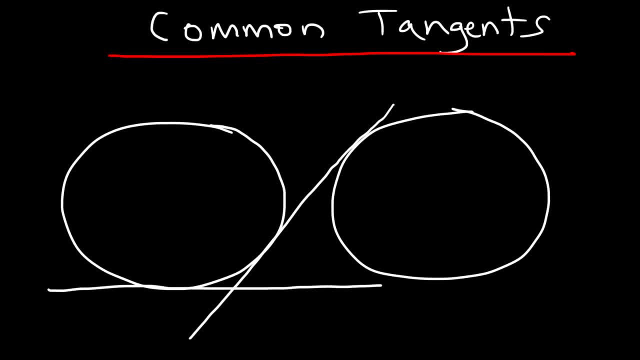 ok, there we go, so let's call this point a and point B. we're going to say that this is point C and point D, so notice that we have two tangent lines. line AB is a tangent line and CD is a tangent line. so AB is tangent to this circle because it only touches the 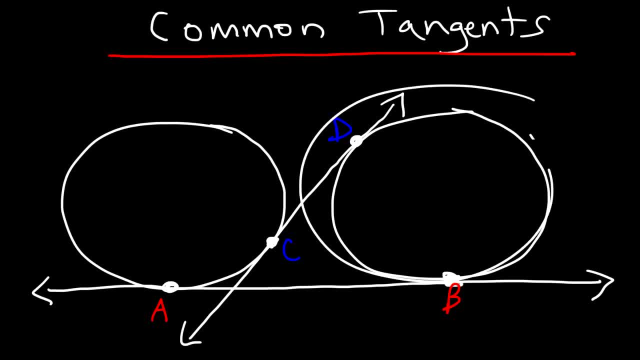 circle at one point it's also tangent to this circle because it only touches that circle at one point, point B. so AB is a common tangent to both circles. let's call this circle e and circle f. this line is tangent to two circles, and so it's a common tangent. 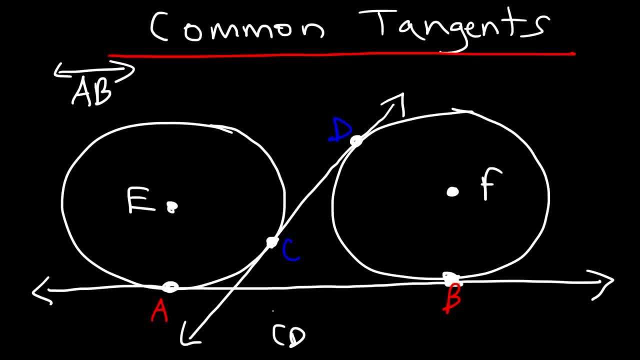 now, line CD is also a common tangent. it touches circle E at exactly one point, which is point C, and it such as circle F at one point, point D. now, what type of common tangent is line AB? what would you say? Now, notice that that tangent line is outside of the two circles, so this is known as a common external tangent. 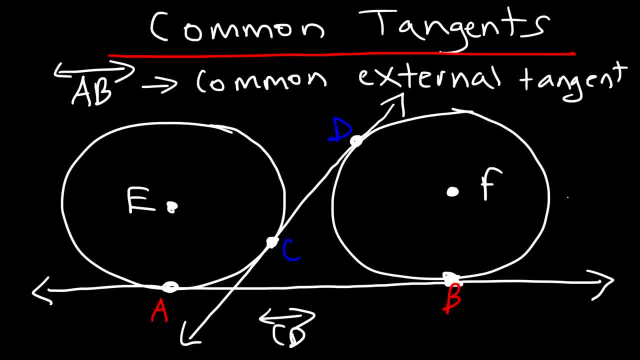 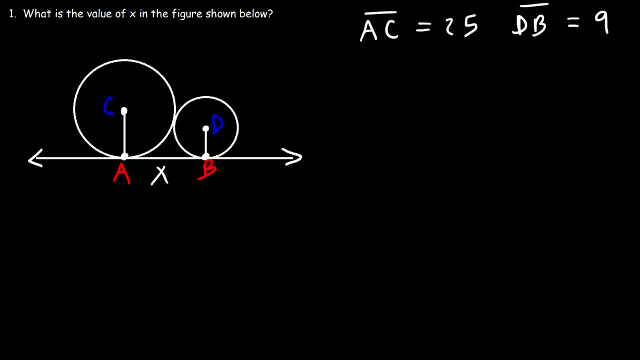 Now notice that line CD is in between the two circles, so CD is a common internal tangent because it's between the two circles. Notice, AB is not between the two circles, so it's an external tangent. Let's work on some problems. So here we have two circles that are externally tangent to each other and we can see that they're externally tangent at this point. 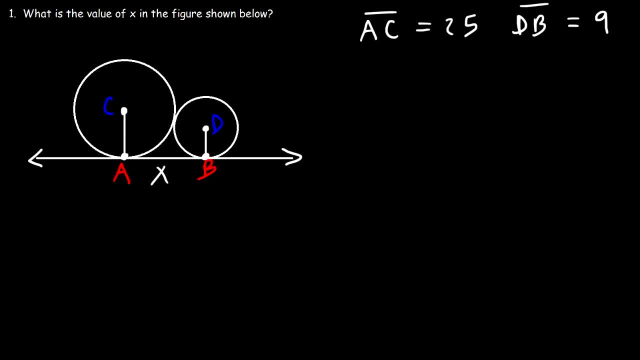 And both circles rest on a common tangent, that is, AB. So what is the length of the common external tangent? The length of the common external tangent, segment AB, which is represented by X. So how can we calculate the length of this segment? So feel free to pause the video if you want to try it. 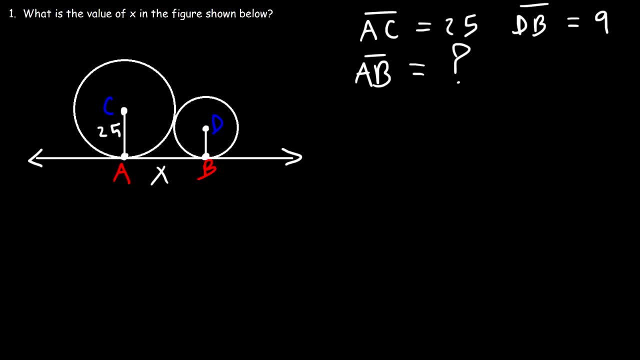 So we can see that CA is 25, or AC and DB is 9.. So let's draw a line that connects point C to point D. Notice that AC represents the radius of circle C And let's call this point Point F. 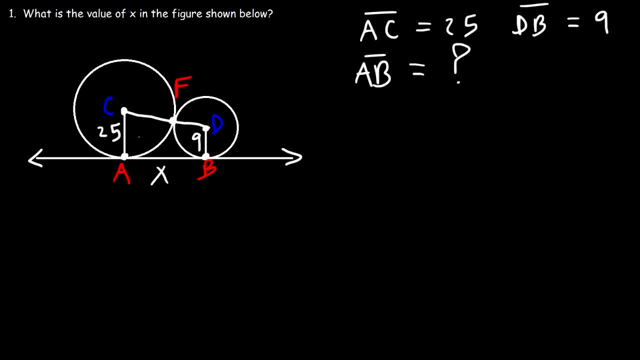 Notice that AC and CF. they both represent the radius of the circle, So CF has to be 25.. Now DB is the radius of the small circle and DF is also the radius of the small circle, So DF is equivalent to DB. 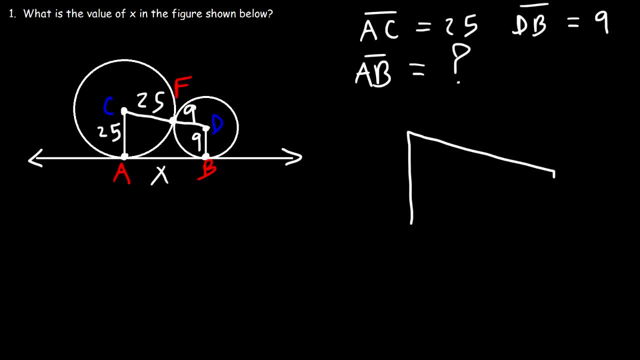 They're both 9.. So now let's draw this figure that we have. So this side, AB, That's X, AC is 25.. DB is 9.. And CD is 25 plus 9, which is 34.. 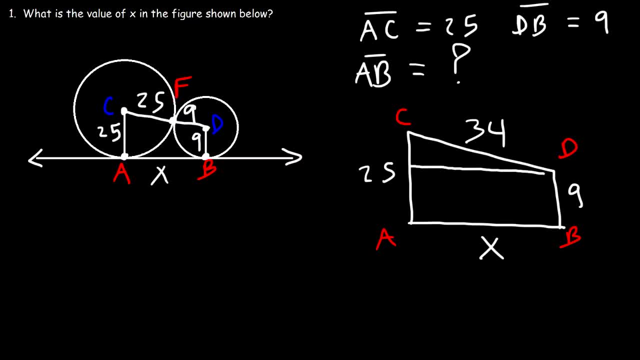 Now let's draw a line that will separate this into a rectangle and a triangle. So AC is still 25.. Now let's call this new point point E. So if we have a rectangle, DB and AE should be the same. So that is, they both should equal 9.. 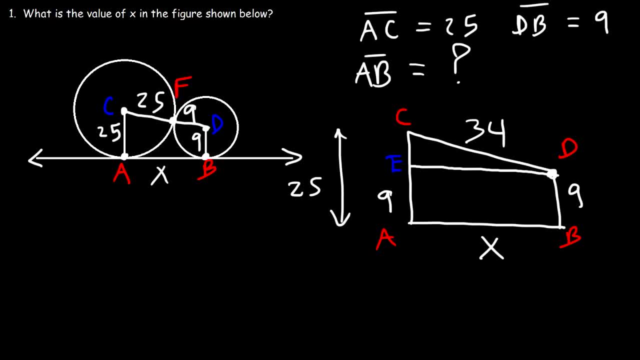 And if AC is 25, that means that CE has to be 25 minus 9, or 16.. So now let's focus on a triangle, Triangle, ECD. So we said EC is not. I mean not 9,, but 16.. 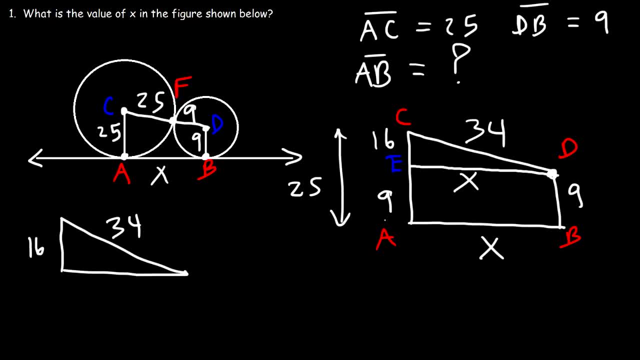 CD is 34.. And DE is the same as X. DE and AB are the same, So now we can calculate the value of X. We have the right triangle. So let's use the Pythagorean theorem: C squared is equal to A squared plus B squared. 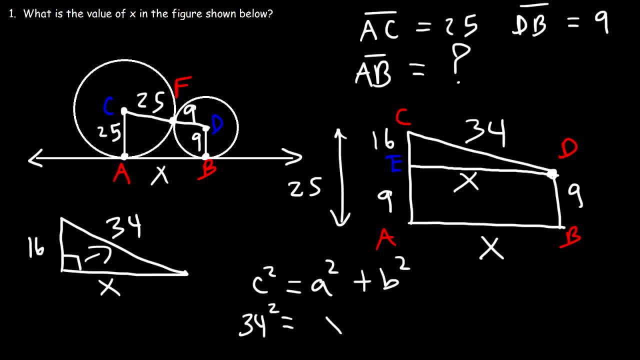 So C, the hypotenuse, is 34.. Let's say A is X and B is 16.. Now, 34 squared that's 1156.. And 16 squared is 256.. So 1156 minus 256 is 900.. 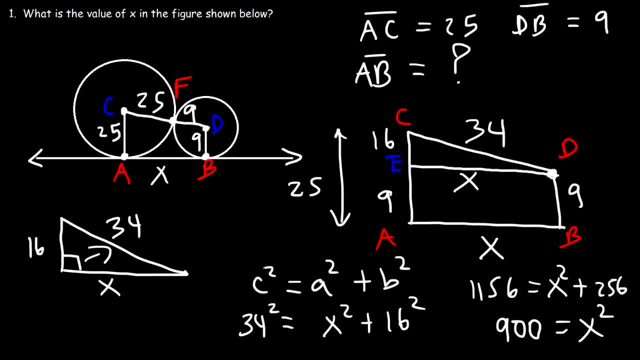 So 900 is equal to X squared. Now all we need to do is take the square root of both sides. The square root of 900 is 30.. And so that's the value of X, And that's what you need to do in order to calculate it in this particular problem. 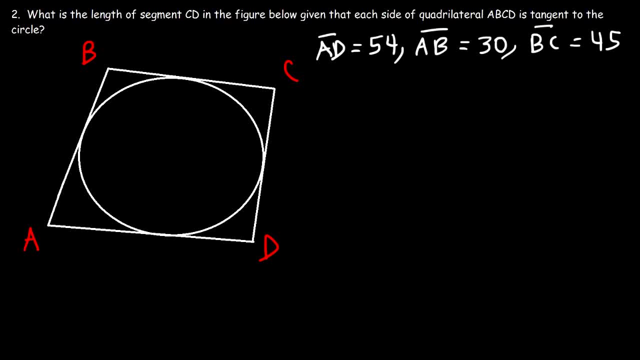 Number two: What is the length of segment CD in the figure below, given that each side of quadrilateral ABCD is tangent to the circle And we're given AD, So AD is 54. And AB that's 30. And we're told that BC is 45.. 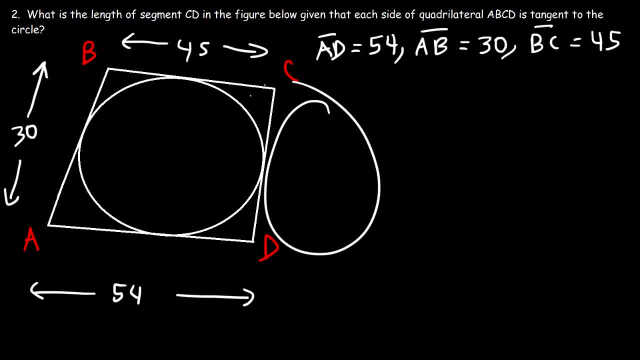 So how can we calculate the value of CD? So let's call CD Y. So what does that mean? What do we need to do? So every side of the quadrilateral is tangent to the circle, So let's label the points of tangency. 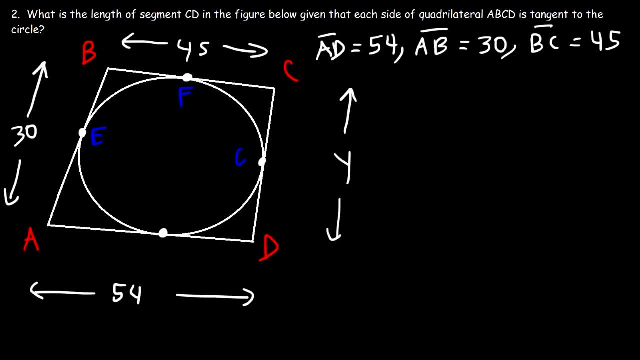 Let's call this point E, F, G and H. Now, in order to solve this problem, we need to understand the principle behind the two tangent theorem, which states that if you have two tangent segments, let's say segment BE and BF. 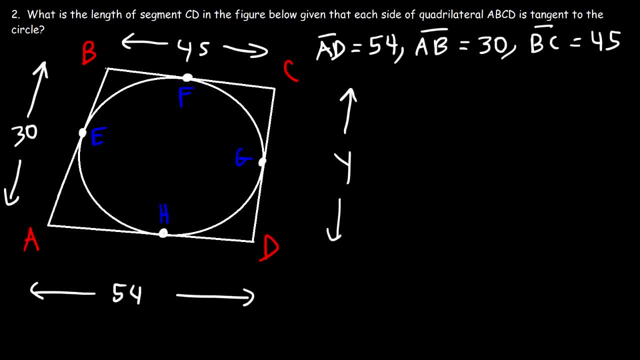 they're both tangent to the circle and they extend from a common endpoint, B, then those two tangents are congruent. So we need to understand that BE and EF they're congruent, AE and AH are congruent, FC is equal to GC. 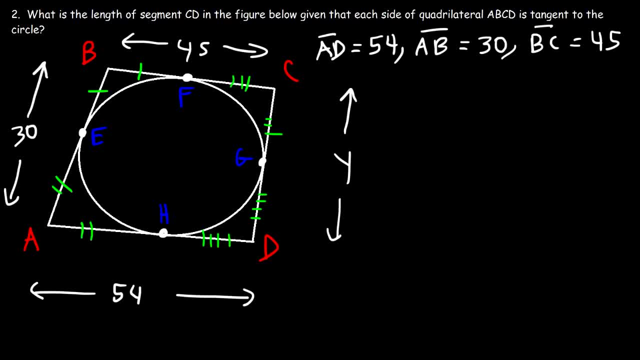 and HD is congruent to GD. So, knowing that if we call BEX, that means BF has to be X. Now, if BE is X, what's AE? This part is going to be the total length, which is 30 minus X. 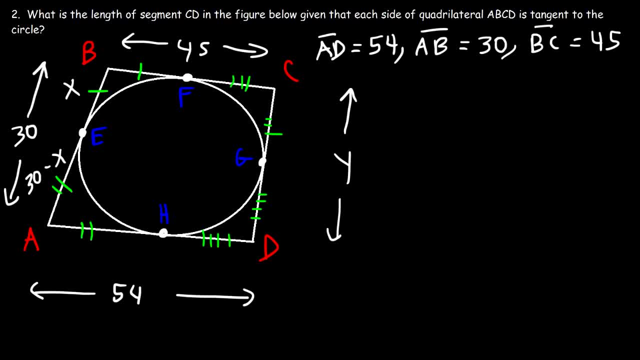 So AE is going to be 30 minus X, And it makes sense because if you add up segment BE plus AE you should get the total segment AB. Now BE is X, AE is 30 minus X. That has to add up to 30.. 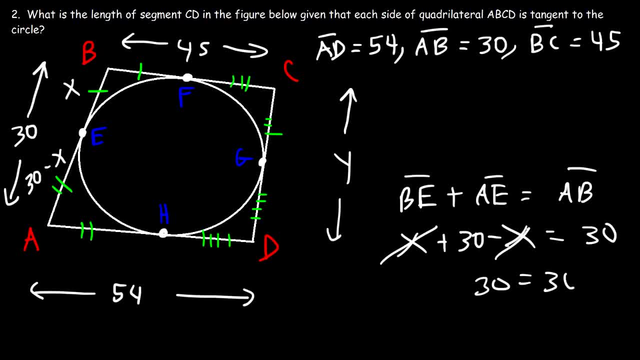 X and negative X, they cancel. So 30 equals 30.. This concept works Now, since AE is equal to AH. AH is also 30 minus X. Now BE and BF they're the same, So BF has to be X as well. 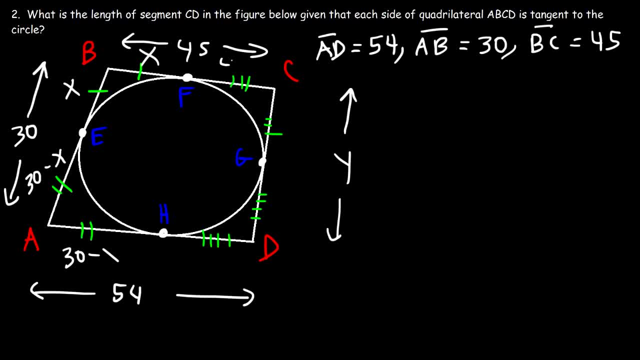 And therefore FC has to be 45 minus X, just as AE is 30 minus X, because X plus 45 minus X adds up to 45.. So if FC is 45 minus X, GC has to be 45 minus X. 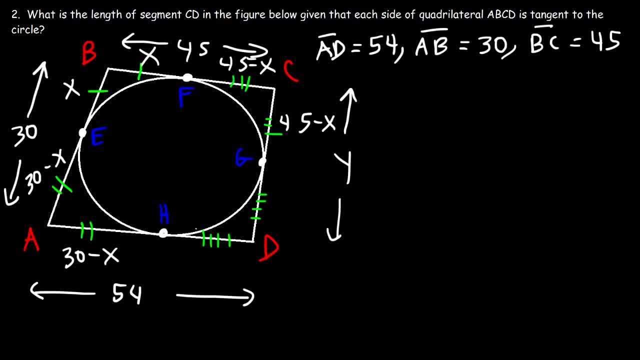 Now what about HD? What is the value of HD? So notice how we got AE based on BE and the total length. AE was just the total length minus whatever this is. So 30 minus X. FC was the total length minus whatever this side was. 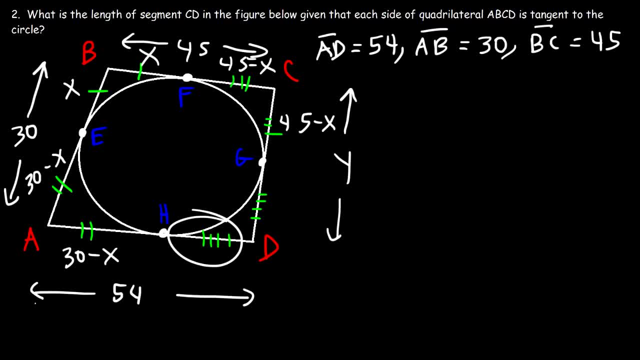 And so that's 45 minus X. So therefore, HD has to be the total length minus whatever we have here, So the total length minus whatever we have here. So the total length is 54 minus 30 minus X. And so, since these two sides are the same, 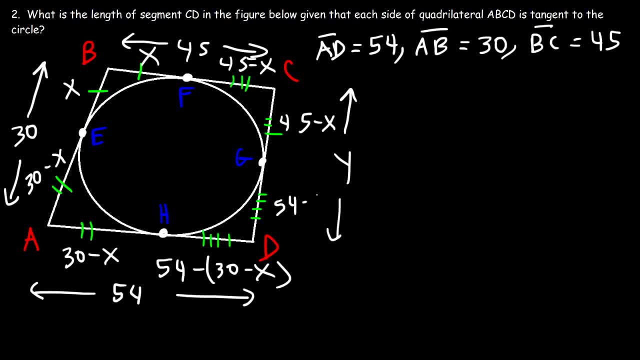 GD is also 54 minus 30 minus X. So now notice that GC and GD adds up to Y, So we can say that Y is the sum of GC and GD And Y represents CD, which is what we're looking for Now. GC is 45 minus X. 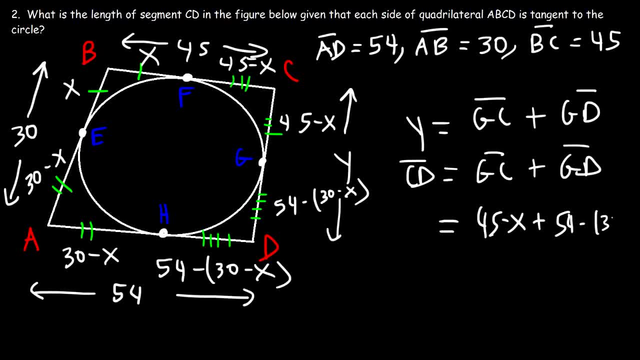 GD is 54 minus 30, minus X, And I'm running out of space. So let's distribute the negative sign, So it's going to be negative 30. And then we have a negative times, a negative X, So that's plus X. 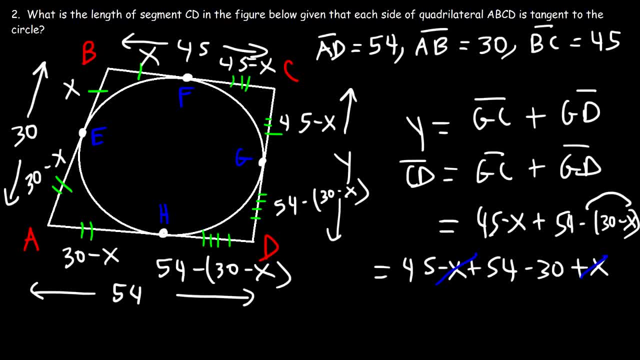 Negative X plus X adds up to 0.. Just as negative 1 plus 1 is 0. And 54 minus 30 is positive 24.. And 45 plus 24 is 69.. So that is the length of segment CD. 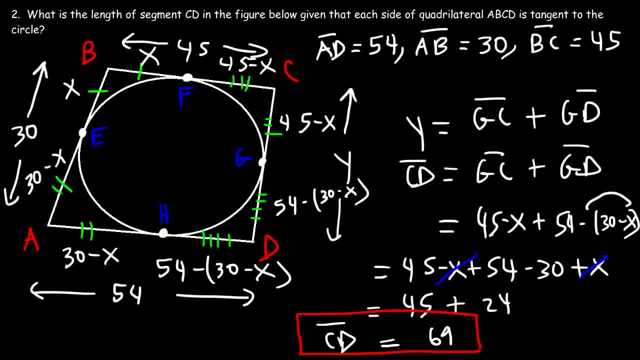 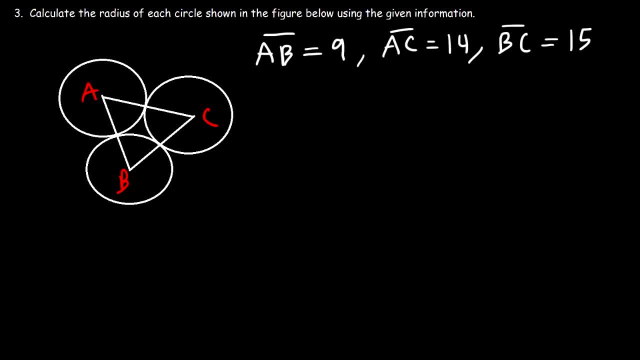 It's 69.. And so that's how you can solve this problem, which is sometimes known as the walk-around problem. Number three: Calculate the radius of each circle Shown in the figure below using the given information. So how can we do this? 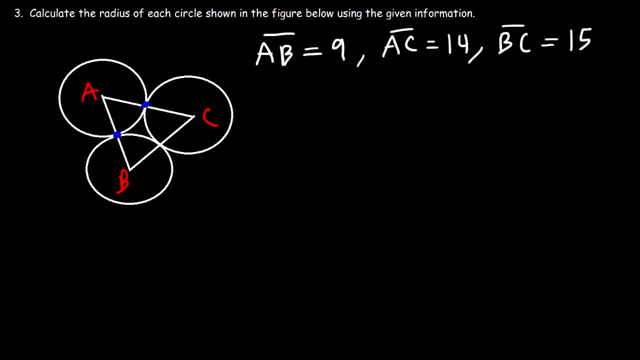 Well, let's label the points where the circles intersect. Let's call this point E, F and G, So we know that AB is equal to 9. And we're told that AC is 14. And BC is 15.. 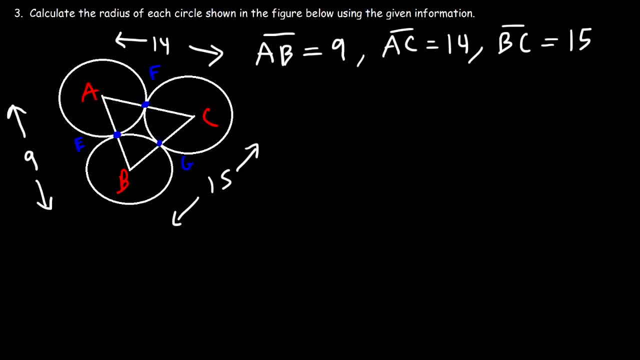 So how can we use this information to calculate the radius of each circle? So notice that AE and AF are congruent Because they represent the radius of circle A. CF and CG are congruent: They represent the radius of circle C, And BE is congruent to BG because it represents the radius of circle B. 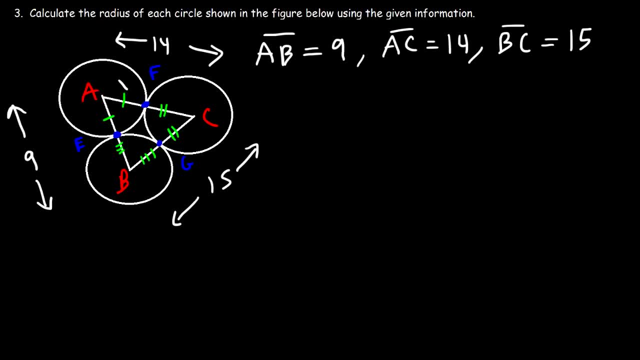 Now let's call AF X, which means AE has to be X, Now BE- this side is going to be the total length minus the other side, So BE has to be 9 minus X, And since these two sides are congruent to each other, 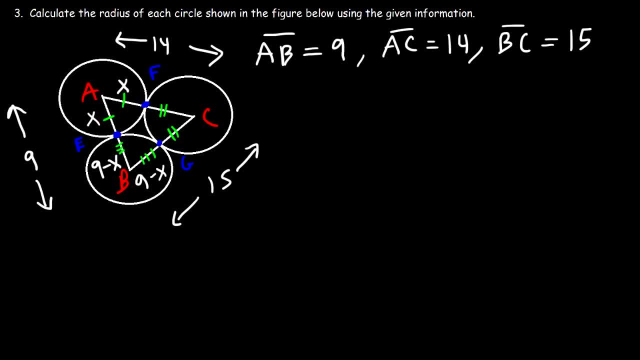 BG is the same as BE, so BG has to be 9 minus X. Now, if this is X and that's 14, the other side is going to be 14 minus X And CF and CG are congruent, so they're the same. 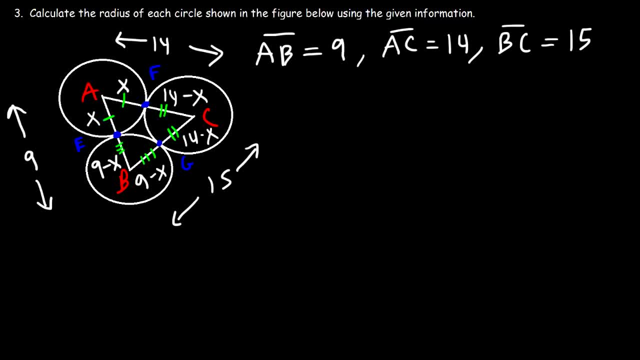 CG has to be 14 minus X as well. Now, BC is the sum of segments BG and GC, So if you add these two, you should get this: BC is equal to 15.. BG is 9 minus X And GC is 14 minus X. 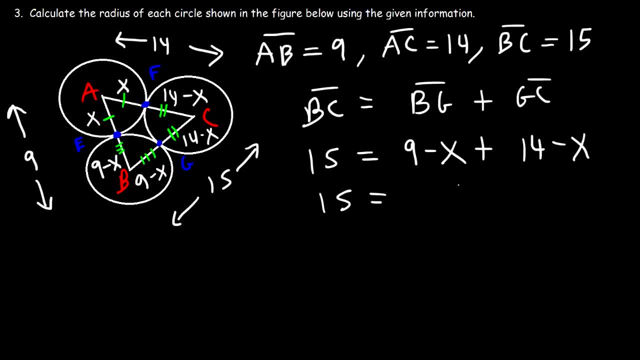 So 9 plus 14, that's 23.. And negative X plus negative X is negative 2X. So what I'm going to do is take this and move it to this side, So it's going to change from negative 2X to positive 2X. 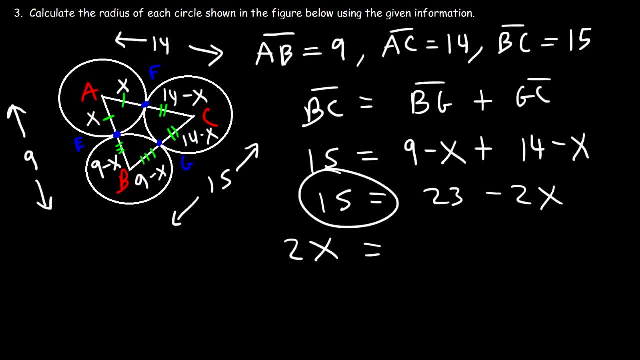 And I'm going to take this number and move it to that side, where it's going to change from positive 15 to negative 15.. Now, 23 minus 15 is 8.. And now we need to divide both sides by 2.. 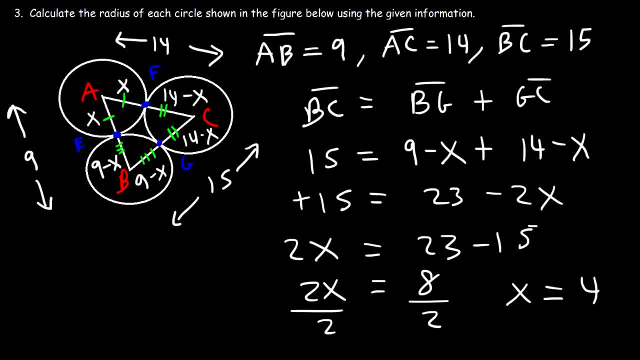 So X is 8 divided by 2, or 4.. So X is equal to 4 in this example. Now we're not quite finished yet, because our goal is to calculate the radius of each circle, So let's start with the radius of circle A. 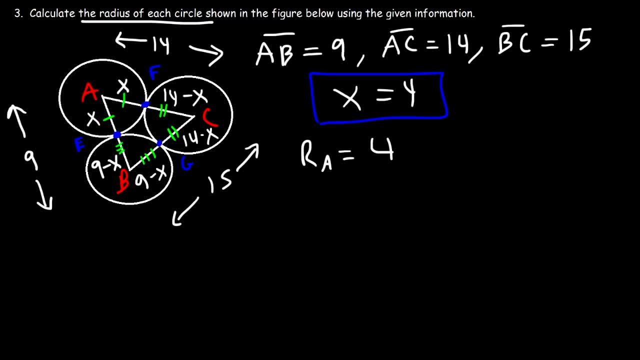 That is equal to X, And X is 4.. So that's the first answer. Now let's move on to the radius of circle B. That's equal to 9 minus X, And so X is 4, so this is going to be 9 minus 4..